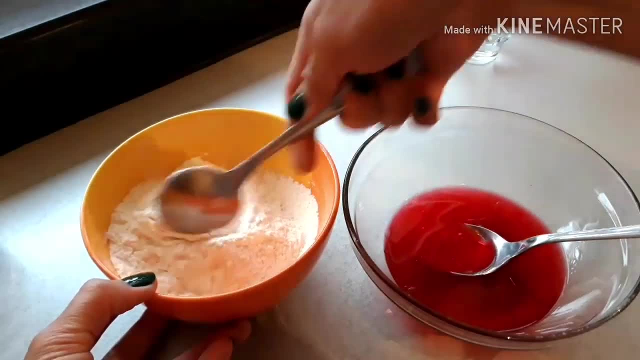 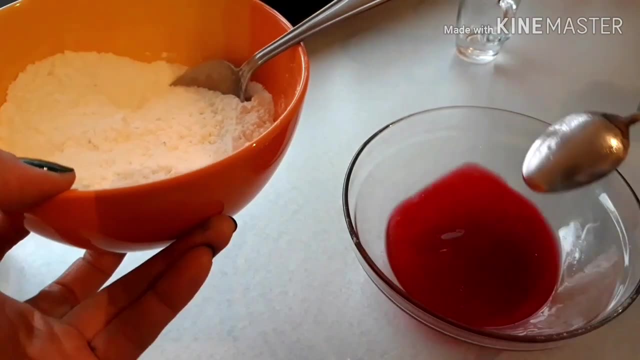 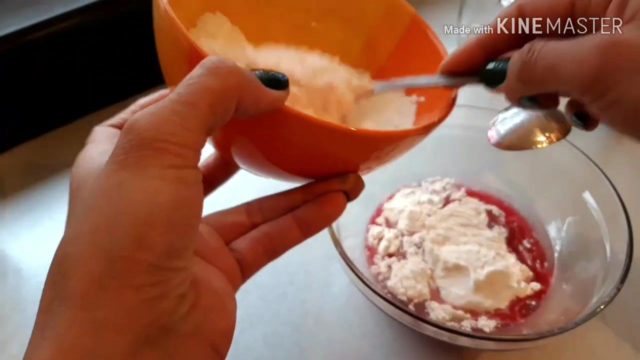 very fast and after that you need put the lid and then it will let it cook more. it will, my will, go to the oven again and I put it here with the�문 and then over it's gonna cook the eggs. put the eggs in something like this and then on the back of your pan. we're going. 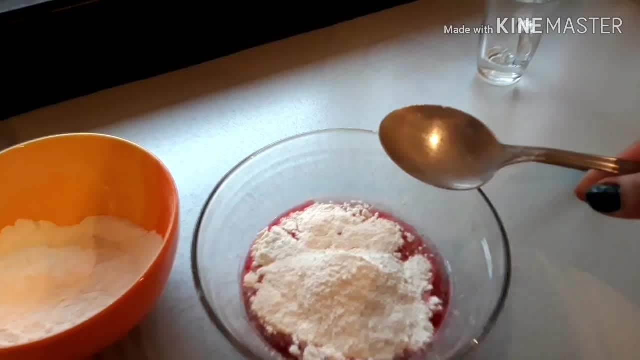 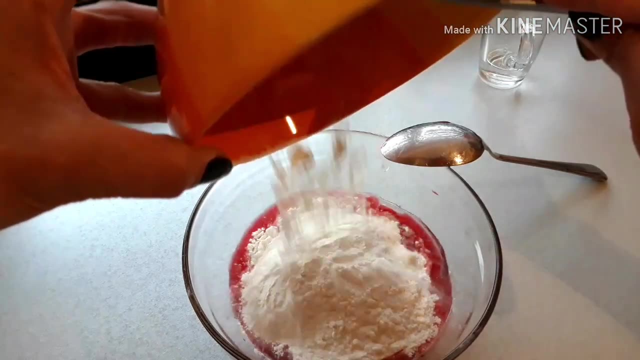 to flip it over. so that's good, we're going to check this process porque we're going to add that one on top of each other. look first and flip it. now. the term I was glad I saw on your channel, not just some mom and not just store things right away, just a. 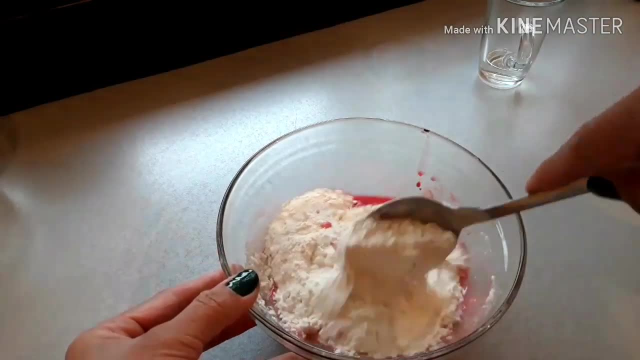 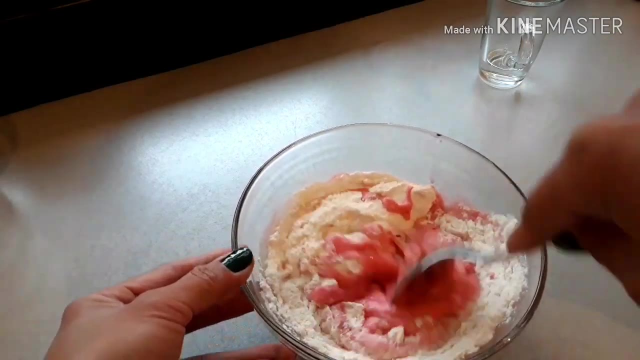 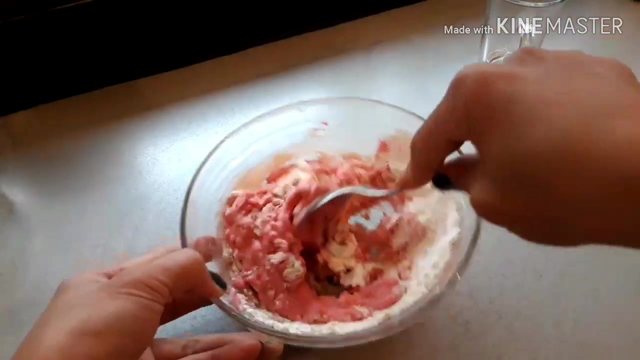 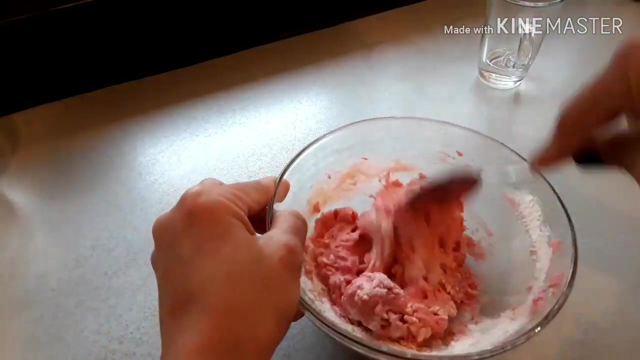 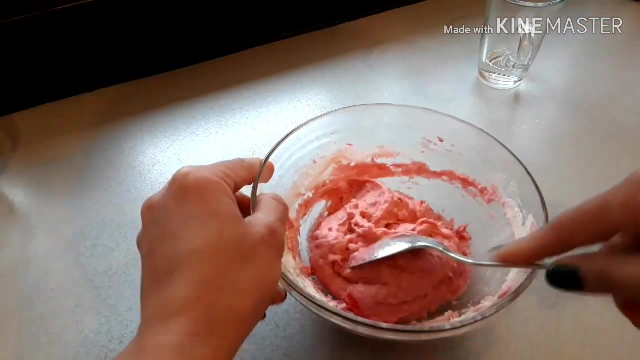 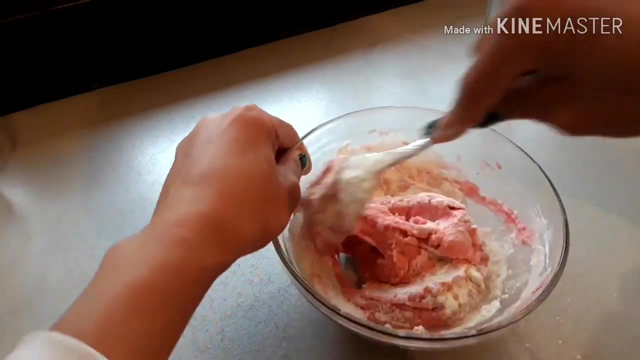 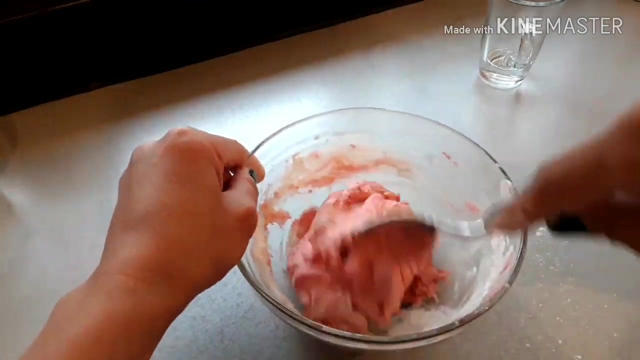 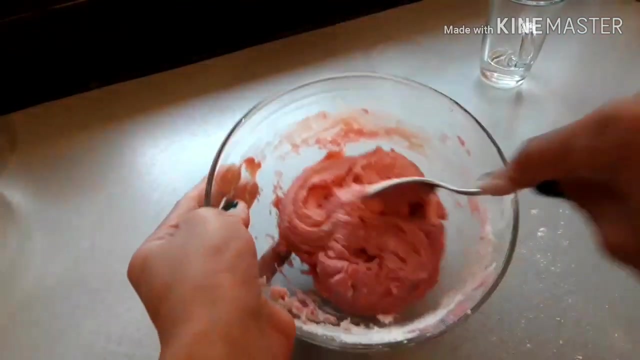 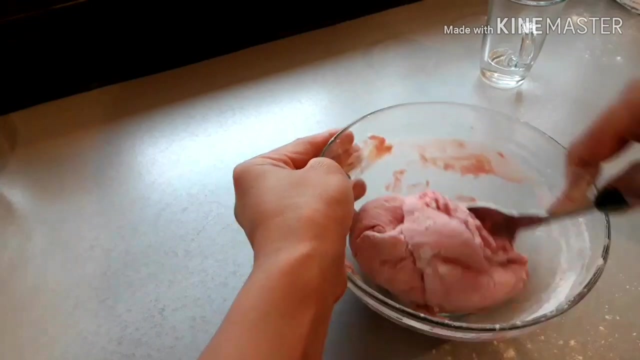 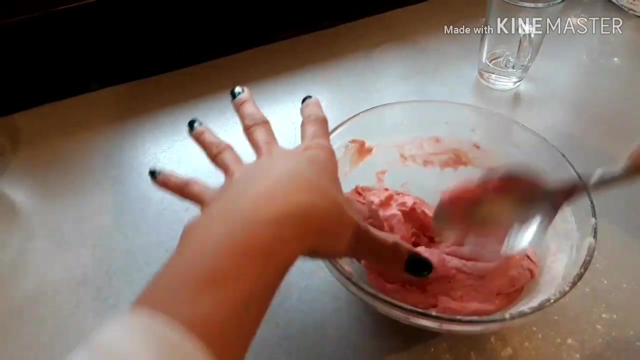 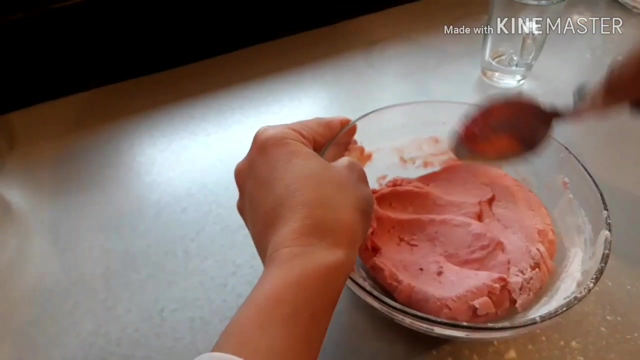 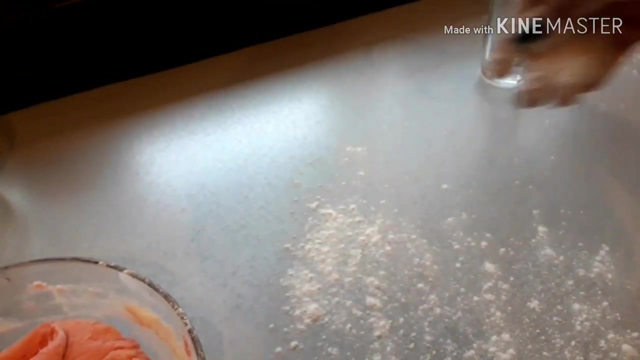 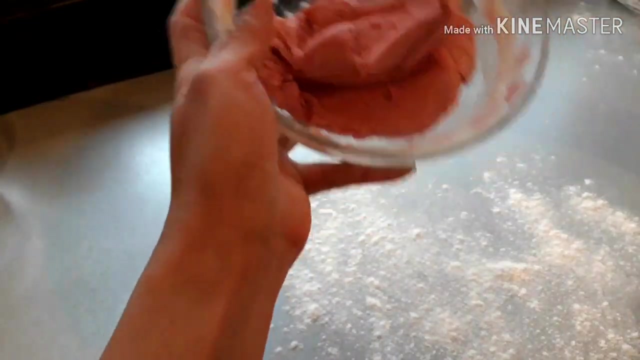 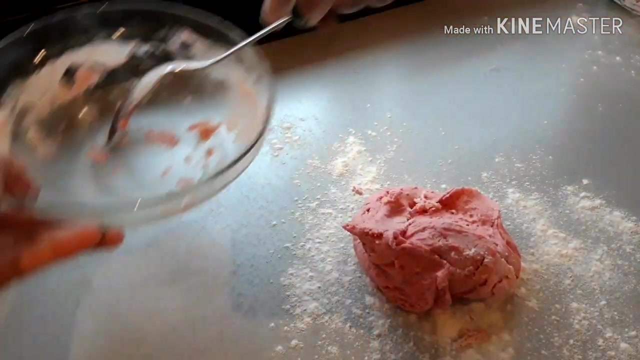 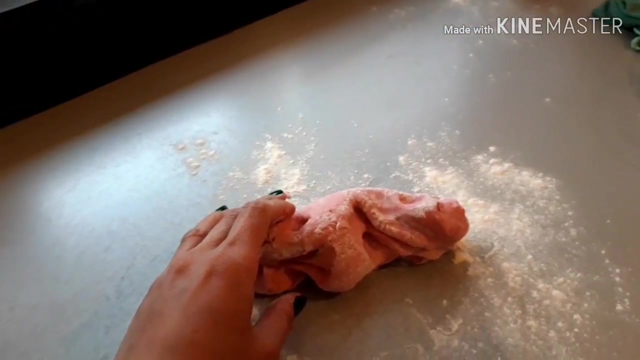 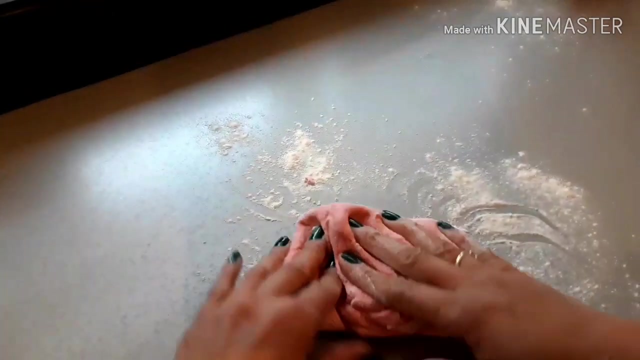 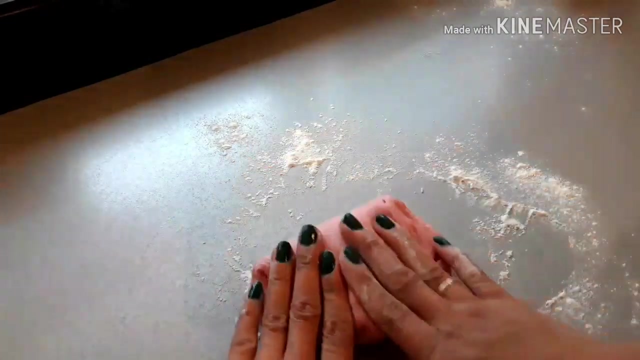 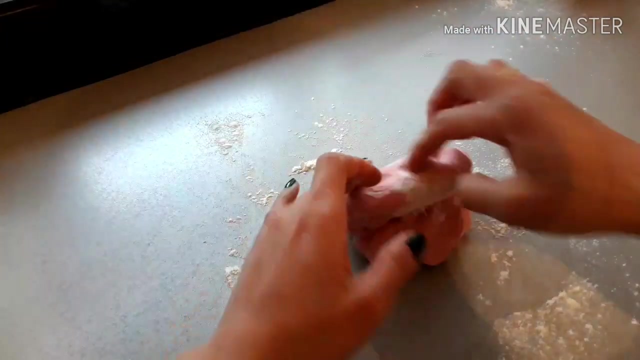 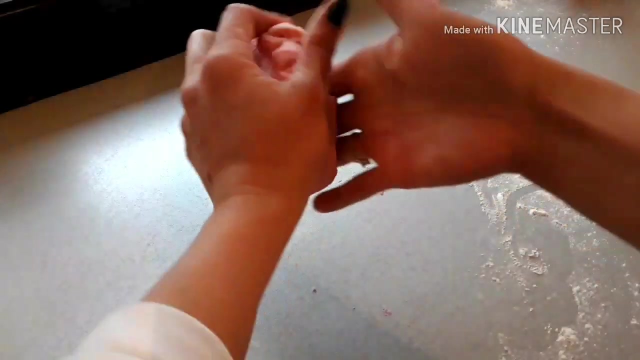 here we go. so you just have to mix it. so, just like that. so it seems a little bit. you see, you can add just a little bit of flour and now we can knead here on the surface. so so, so, so, so it's just so easy, guys.